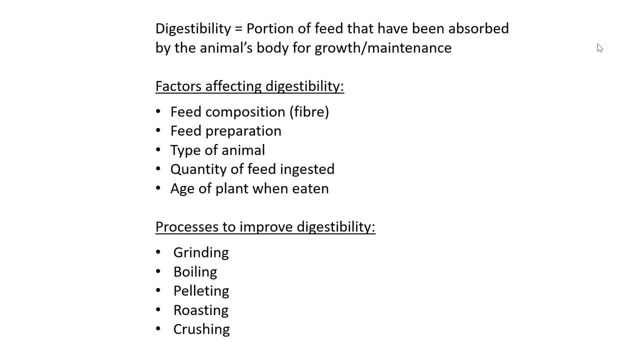 specifically for either growth or maintenance, And I just want to mention that there is a difference between growth and maintenance. So growth usually has to do with, like your young animals, they're still growing, still building muscle, they're gaining height, Whereas for maintenance, this is just, it just keeps the animal alive. So usually when a farmer 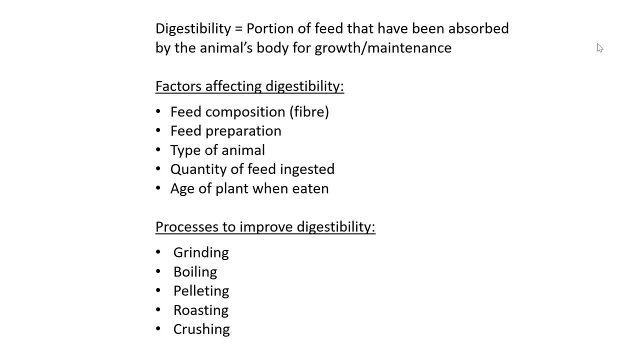 gives feed to an animal for growth purposes, he has to give over and above what the animal actually needs, So he has to give extra. that, while it's still growing, won't necessarily become fat in the animal, but it will actually help it build muscle and grow and become taller. 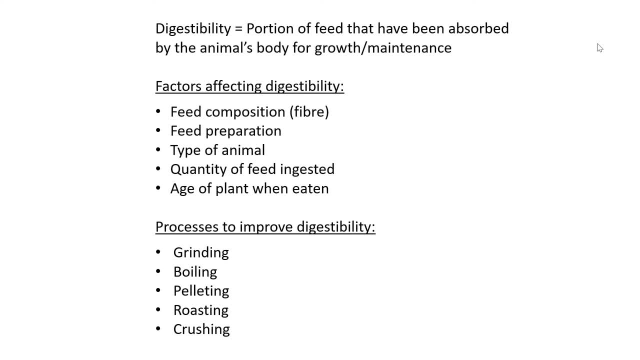 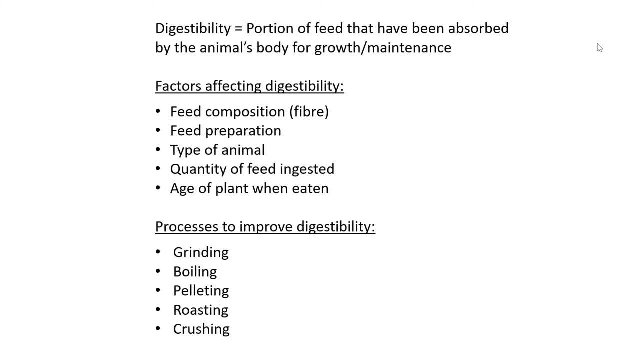 them too much, otherwise they become fat. So you just want to give enough to keep them in their current condition and keep them alive. Okay, So then there are a couple of factors that affect your digestibility. The first thing. first thing is like your feed composition. So is there fiber? 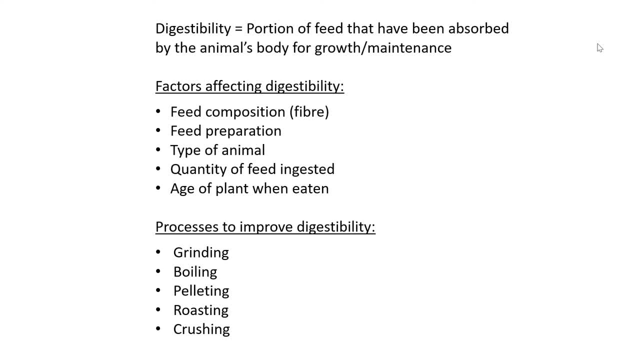 in the feed? Is it just plain protein carbs? What are you giving them? Secondly, which affects how good they absorb the feed is the preparation of it. Was it just felt you allowed the animal to eat, which has a lot of fiber and cellulose and tough materials? 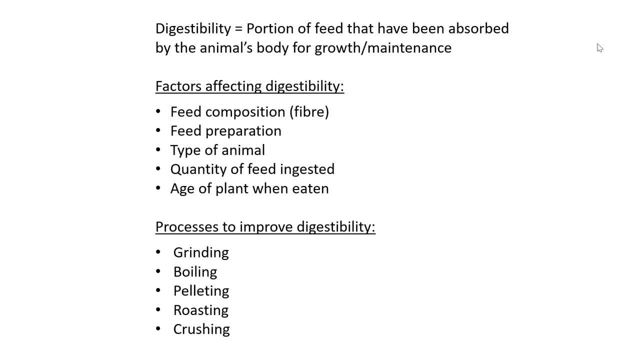 or was it actually prepared by soaking the feed in water, or did you boil it, or did you do something to it? Thirdly, the type of animal. some animals absorb feed just better than other types of animals. Then also the quantity of the feed. did you give it enough? Did you give it too little? 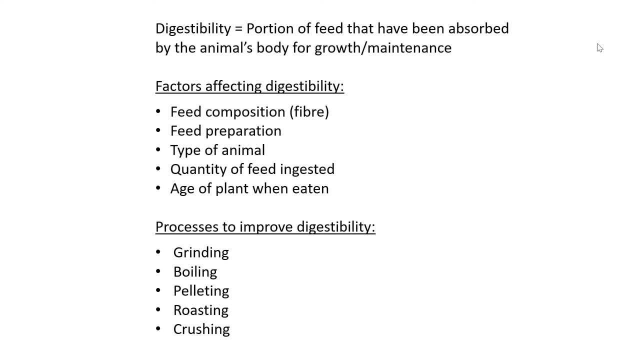 too much? That's a good question. So the quantity of the feed: did you give it enough? Did you give it enough fiber type thing. Then the age of the plant when eaten. So usually your young plants, especially when they're still soft and tender, they digest much, much quicker and easier than 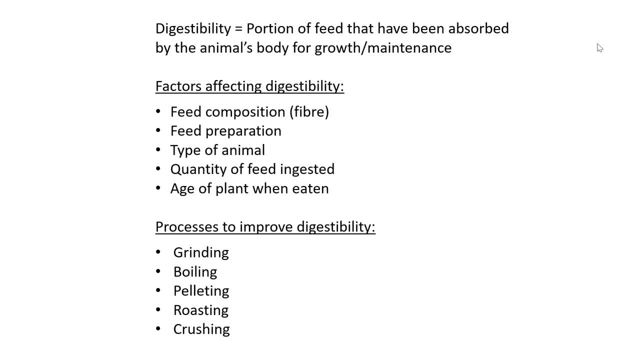 your tough cellulose, thick plants. So it depends on the age of the plant usually. And lastly, for farmers, how can they actually process the food they give the animals? to improve the digestibility of the feed, There are a couple of things. You can grind the feed. Think of corn. 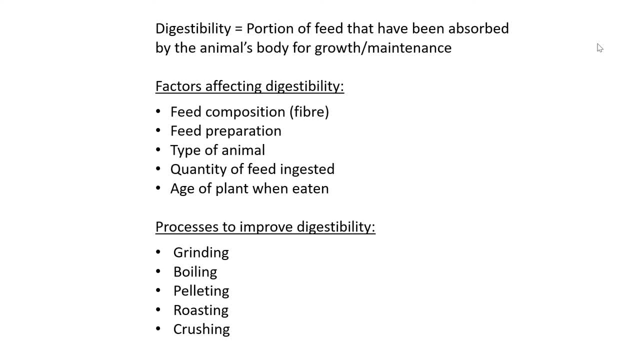 usually it's ground to make it a little bit more fine. You can boil, you can feed, you can pellet it. So little pellets to make it especially for chickens. they love picking up the pellets And then roasting it, probably usually with roasting. 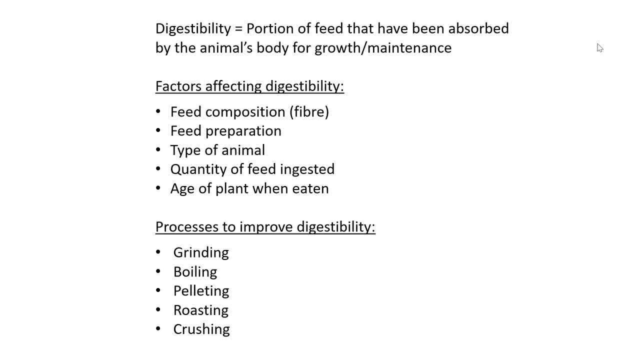 you break open the outside- let's say it was four seeds or something you burst roasting bursts open the outside husk of the seed and then it's better for the or easier for the animals to get to the inside, which actually has all the nutrients. 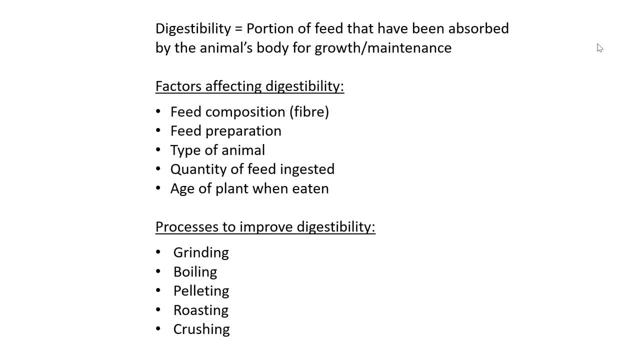 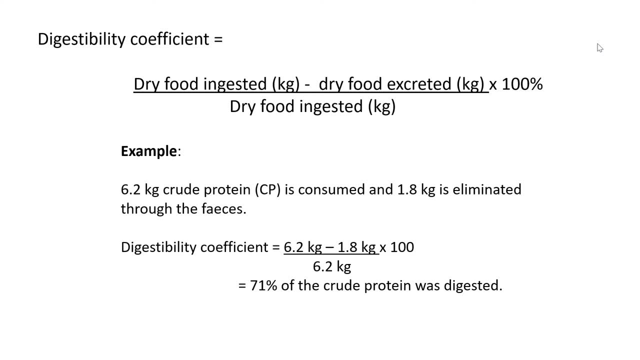 And then also crushing feed to make it maybe into a meal format or a flour format. Okay, so from here on we're doing a couple or a lot of equations and mathematical things, so that we have to do a couple of calculations. That's the word I'm looking for. So the first thing is the 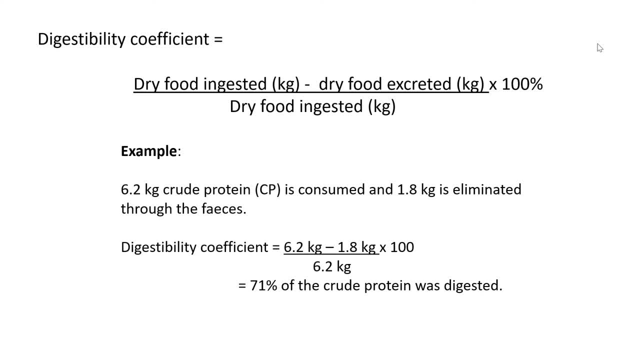 digestibility coefficient. So this is a mathematical way of figuring out what you have given the animal and whether the feed actually went into the animal, whether the animal absorbed the feed. So the equation here is very important. They do not give the equation. 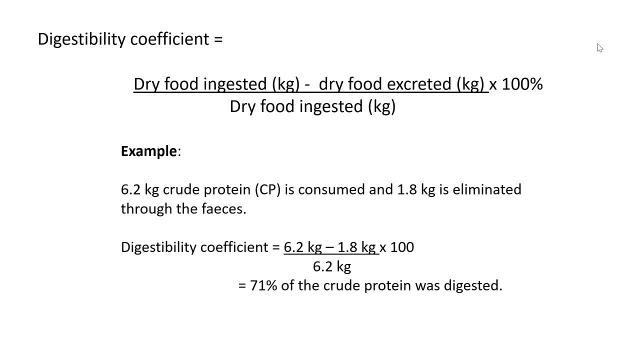 in the exam. you have to memorize this out of your head. So the equation here is: dry food ingested, whatever the amount of kilograms you gave the animal, but it must be dry, minus the dry feed that was excreted in the manure, also in kilograms. Divide that with the dry food that was eaten. 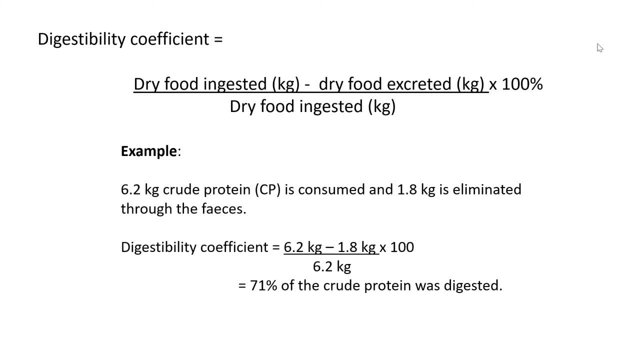 and times it with 100. So the coefficient is going to be in a percentage. So here's an example: 6.2 kilograms crude protein. Don't worry about the fact that there's protein or fiber or whatever, but the fact is we know the animal was given 6.2 kilograms of feed to eat, So it consumed it and 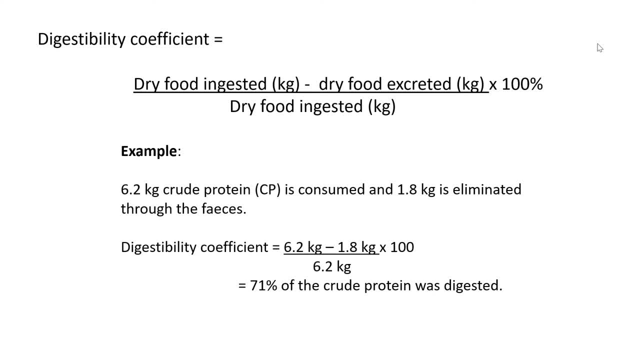 then 1.8 kilogram was eliminated in the feces. So put that just into your digestibility coefficient. It is 6.2 kilograms minus 1.8, because you don't want to know what it excreted, You want to know what actually absorbed. So you have to minus what was eliminated out of the body. 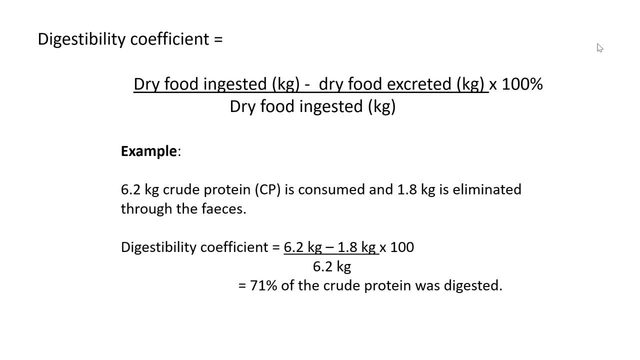 And you divide it by 6.2 kilograms, which is the total times 100. And then you get 71% of the crude protein was actually digested. So what this means is that 71% of the crude protein the animal actually took in or ate was absorbed in the body. So this is actually a good thing. 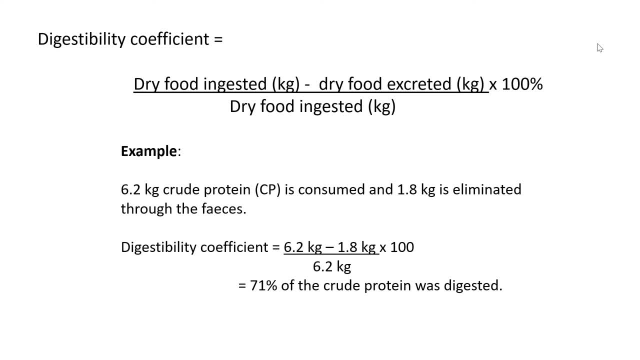 It's a good value. It's a higher value, much higher than 50%. If that percentage was something like 20%, it is a reason for the farmer to panic because that means everything- mostly 80%- was excreted out of the body with the manure. So the fact is the farmer would be losing money. 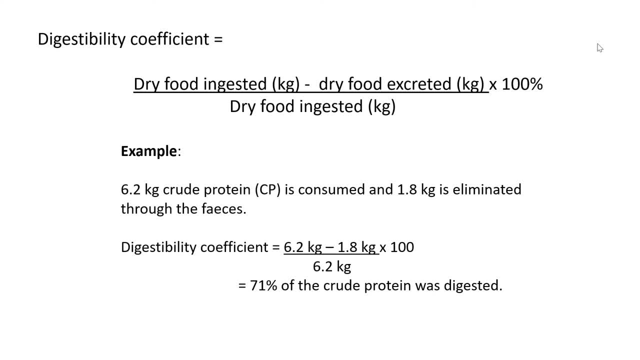 But the fact that it's 71% of the crude protein was actually digested. so what this means is that 71% that was absorbed is a good thing, So the animal actually gained some feed and nutrients. Hopefully it's still growing or it can be used for maintenance. 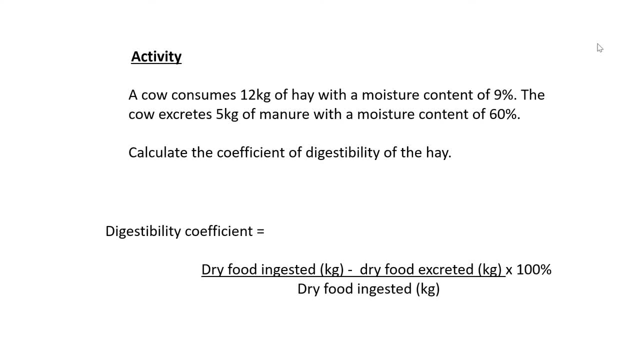 So here's just an activity I would recommend at this point. if you want to do on your own, Pause the video, because the next slide will give you the answer. Okay, so in this case, a cow consumes 12 kilograms of hay, but there's a moisture content. 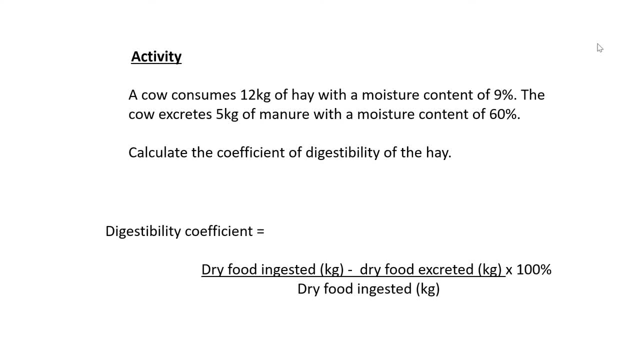 And in the equation, the bottom here, it says it wants dry food ingested and dry food excreted. So you have to figure out: if 9% is the wet feed, obviously what's going to be the dry feed. Okay, Then they also give the cow excrete five kilograms, but that is what: wet manure and 60%. 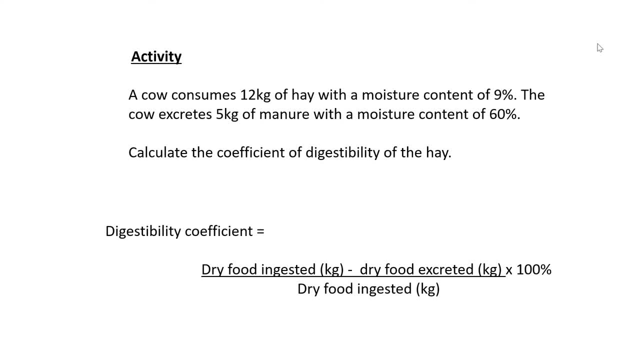 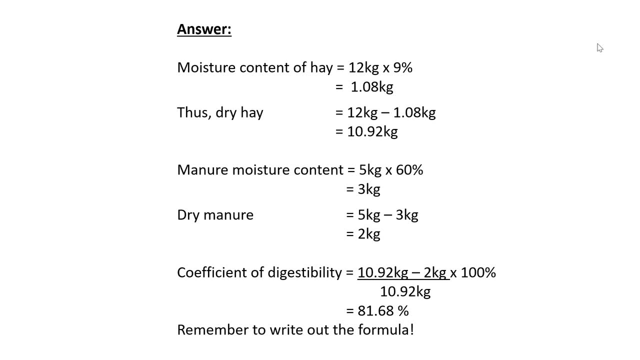 of it is wet, How much of it will be dry? Okay, Then you have to calculate the coefficient. So here's your answer. Firstly, because it's the long way you could have. instead of saying well, saying 12 times 9%, you could have said 12 times 91%, because 100% minus 9, that gives you basically. 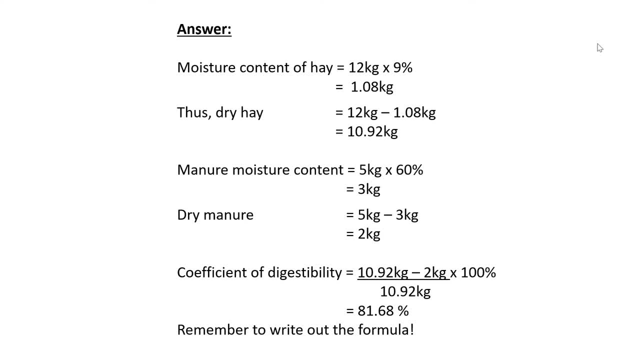 the dry feed, And then you will already get, or come to, 10.92 kilograms. So this, basically, is your dry feed. This was feed that still had moisture in it. Okay then for the manure, the same thing. you could either have used 60% or 40. If you said 5 times 40,, you would have come to 2 kilograms. 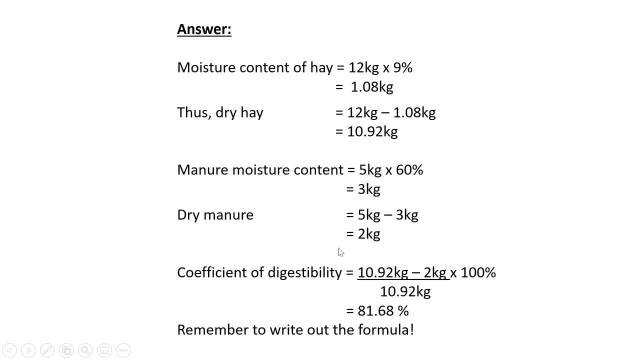 So then you just have to substitute all the dry stuff in, So for your coefficient 10.92 kilograms minus 2 kilograms dry feed, dry waste, divided by the dry feed that was ingested, so the total of the dry times 100%, And then you get 81.68%. So this is also a very, very high percentage, or? 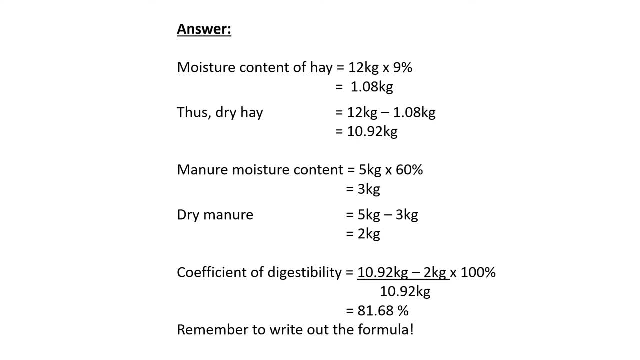 coefficient, which is good. So 81% roughly, or 82%, was absorbed by the animal or the nutrients. And just a reminder: please remember the formula. You guys get a mark for the formula for just writing it. So in this case I didn't have enough space So I did not write the equation out in. 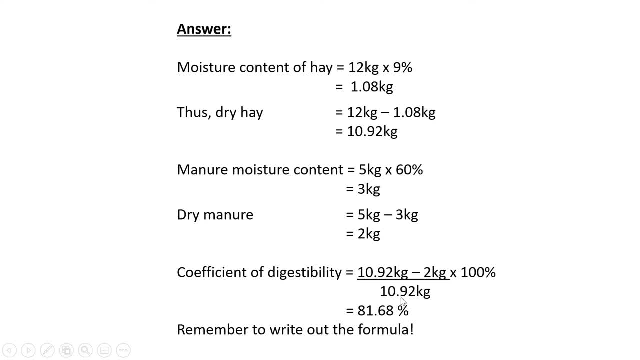 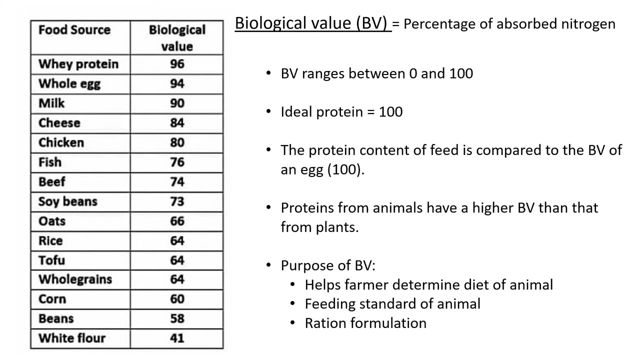 words. But you get a mark for that, Usually two marks for this, for substituting everything incorrectly, And then one or two marks for the answer and saying percentage. Okay, so then we look at the biological value. So the biological value itself is the percentage of. 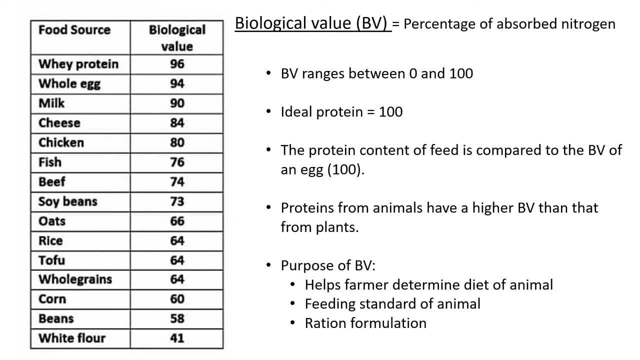 nitrogen. So the previous one was just to figure out how much nutrients was absorbed, But now the biological value focuses on the protein itself, or, well, everything that has nitrogen, which is basically your protein. So I just want to mention that the BV value, or the BV, usually ranges between: 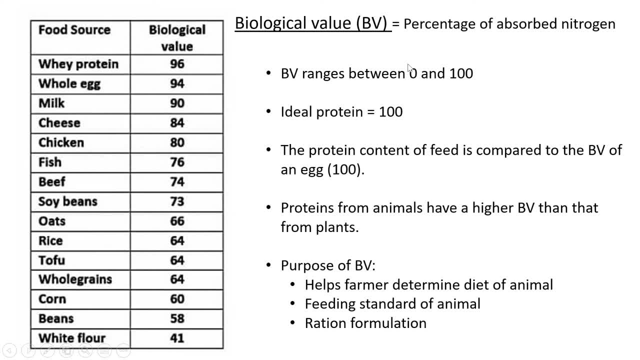 zero and 100.. So meaning there is zero nitrogen amounts of nitrogen in a feed or there is 100%, technically percent in the feed. So the ideal protein then would be 100.. So the highest the beta. So here: 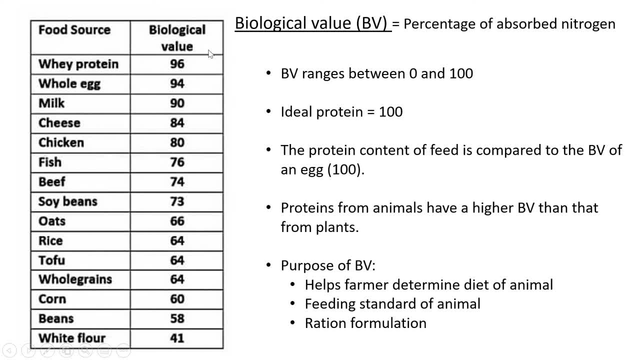 I just want to digress and go to this side of this table. Here we can see that whey protein in a whole egg is very, very high, So it's 94, 96.. Usually they say an egg has a value of 100. 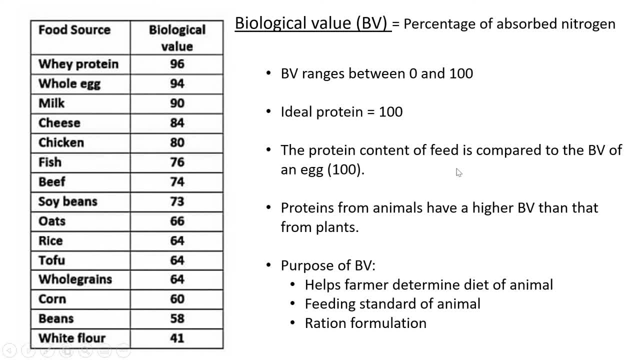 Like here, the protein content of feed is usually compared to the BV of an egg, which they say is 100.. Technically it's not 100. But since it's so high, so high in the 90s, usually scientists 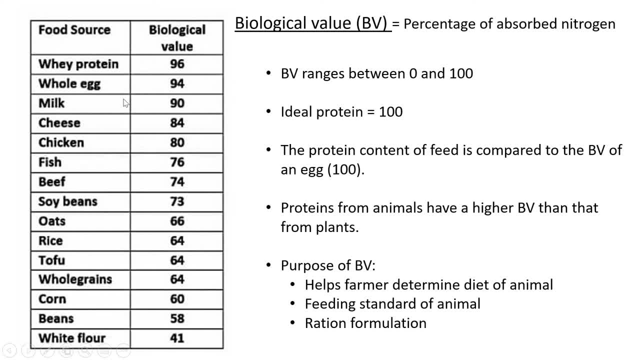 assume it's 100.. Okay, so things like a mock egg protein, a whey protein is like protein flour or yeah, yeah, basically protein is very, very high. So all the BV value basically what it does is it compares any food type you the farmer wants to give to its animals. 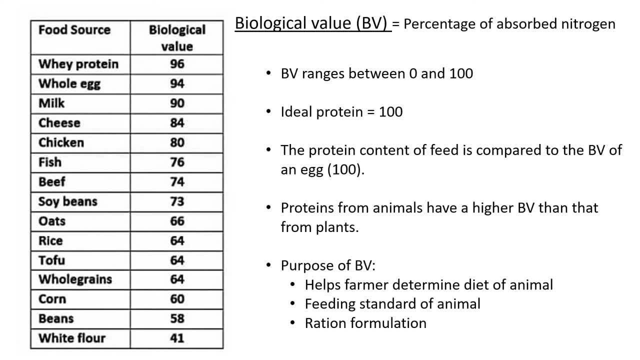 It compares its nitrogen content with the nitrogen content of an egg, because an egg almost has 100.. So that's your ideal protein you want to give, or the ideal food source. So on this chart you can see that the BV value is 100. So that's your ideal protein you want to give, or the ideal food source. So on this chart, you can see that the BV value is 100.. So that's your ideal food source. So on this chart, you can see that the BV value is 100.. So on this chart, you can see that the BV value is 100.. So 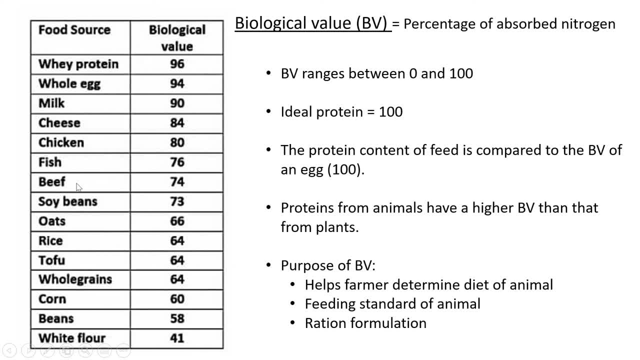 here is your animal feedstuffs or animal products. They have a high BV value, so a lot of nitrogen, a lot of protein. But plant based things like beans, oats, rice, corn, beans have exceptionally lower amounts of nitrogen. So point being here when farmers have to give or supplement their 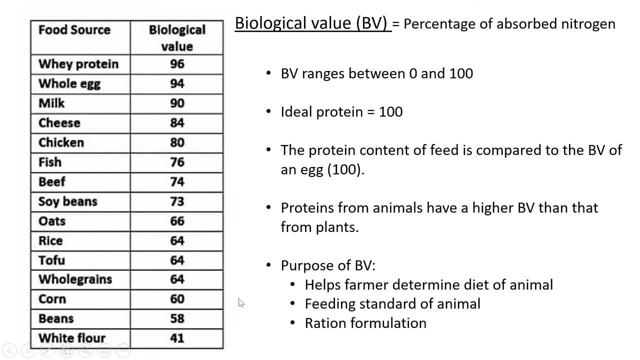 feeds to their animals and they want the animals to gain more protein. they have to give animals animal-based protein or food sources to the animals. Then they get a lot of nitrogen in. So proteins from animals have higher BV than that from plants, just said. And lastly, what is? 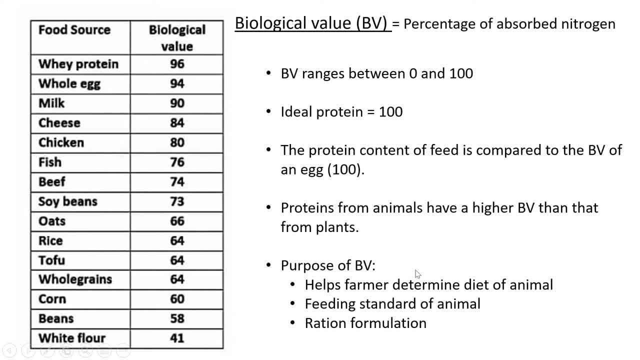 basically the purpose of the BV. It helps the farmer to determine the diet of the animal. So again, they want to make sure that whatever the animal is eating has enough protein in And the farmer can figure out the diet and figure out whether the animal needs extra nutrients or extra. 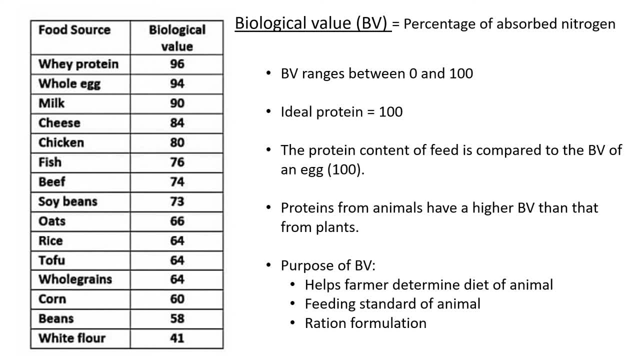 supplementation, Then secondly, feeding standard of the animal. So again it actually goes with the first bullet to figure out whether the animal is eating or what it's supposed to be eating, getting in the right nutrients it needs for either maintaining the animal or for the animal to still. 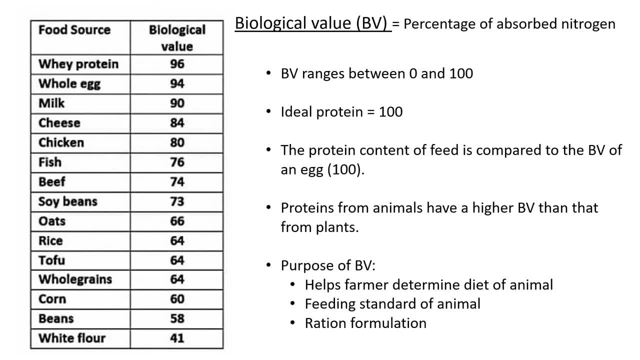 grow And then last. it also helps the farmer for ration formulation. Basically, all three of these bullets have to do with the same thing. The farmer has to figure out whether he needs to supplement. Can he just give the animal roughage, which is basically them eating? 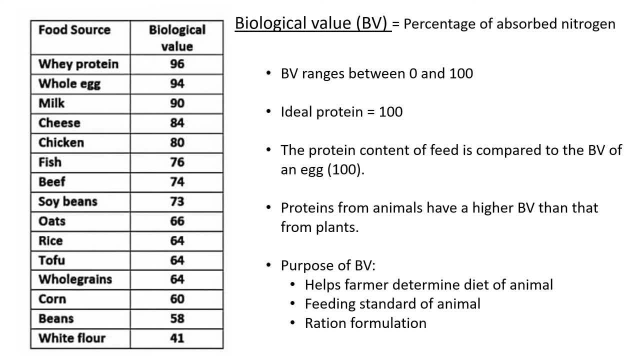 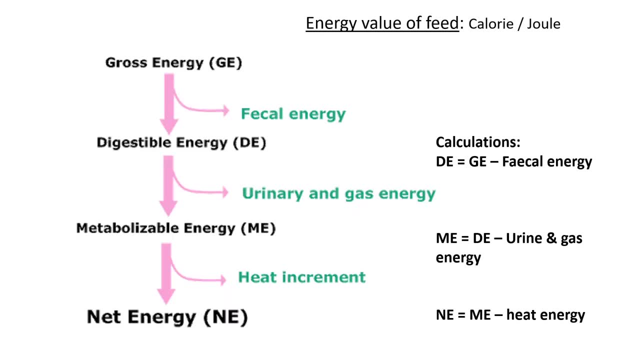 off the felt, Or is it needed to give them extra concentrates, which could be like molasses, which has more sugar in it? Does he have to give more carbs or anything else? More vitamins- Is there deficiency somewhere? So that has to do with that. Okay then I just quickly want to mention 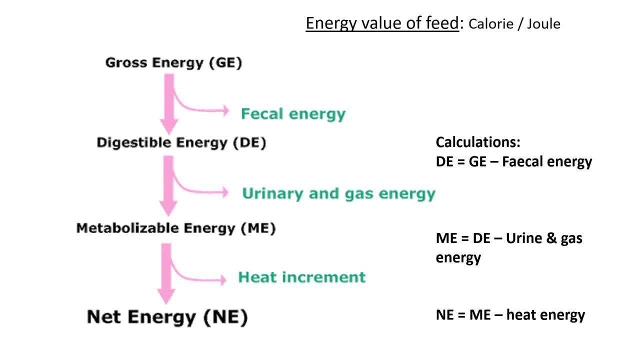 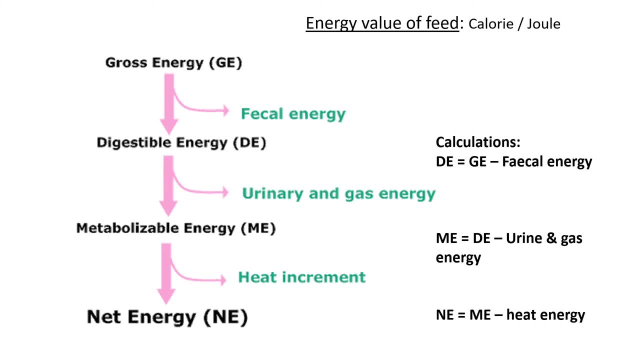 you know we measure it in joules, Unless your body needs to keep rehydrating, rendezvous or training. And so do we measure it in joules, because what's been measured is okay. there must be a particular 95% cultural weight of nourishment content, and I guess that kinds. 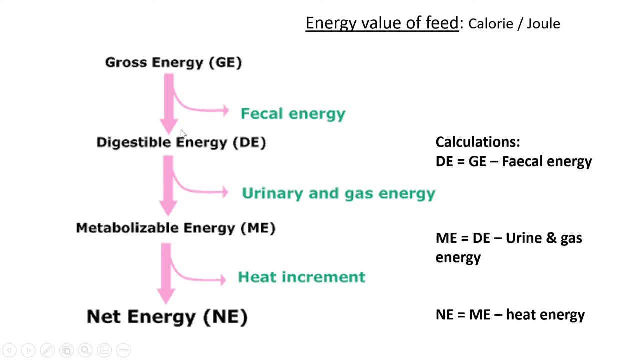 offight in the becoming plants that produce those influenced nutrients, and there's a�isty thing that they're energy and also body agents and so on, which is interesting. energy, Then, at a stage while metabolism is happening inside the animal's body, and so on. 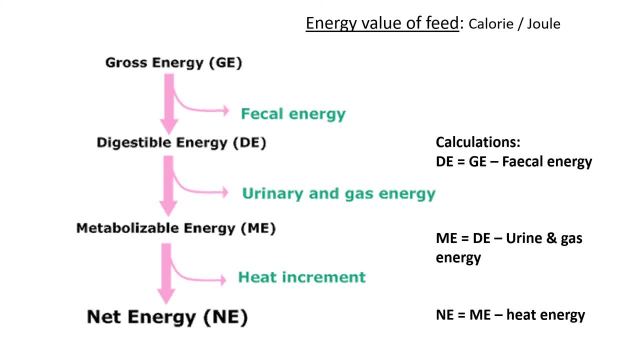 some energy that the animal has absorbed goes out the body with the feces. So when you have the gross energy and you minus the energy that was lost through the feces, it is called the digestible energy. So to get the digestible energy, you say the total energy which is the gross energy. 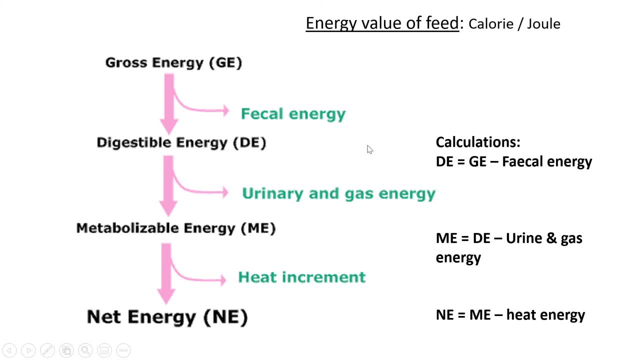 minus fecal energy, Simple enough. So that's how you get the DE And they usually use G-E-D-E-M-E-N-E. So you have to memorize the shortened version So you don't have to say gross energy every time or digestible energy every time. You can use the shortened way of saying it. 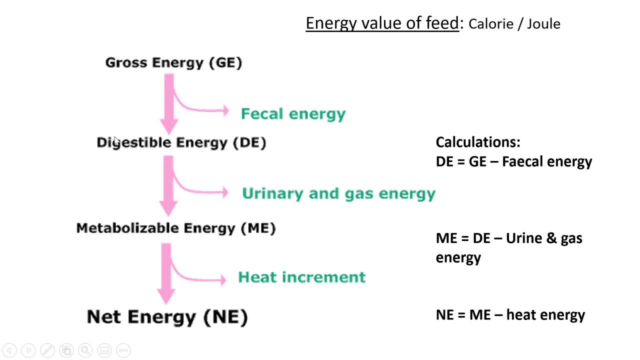 Then when you have your digestible energy, some energy will also be lost through the urine of the animal and gases of the animal. So meaning some after- especially for a cow- after the microbes have digested, or helped them digest, cellulose and lignin and all these tough. 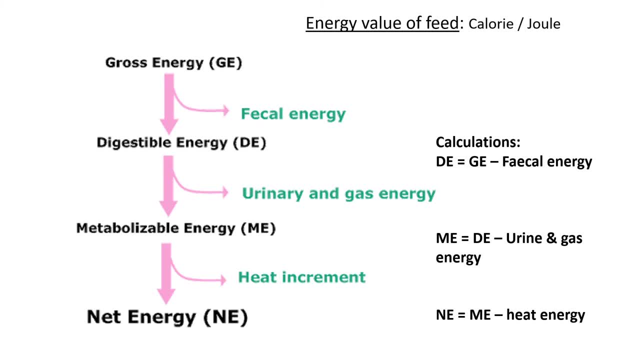 plant materials in their stomachs. they emit methane gas out their bodies, So it also releases heat into the atmosphere. So that gives us: when you've eliminated these two heat sources, you get. they talk about metabolizable energy, but a better word would be metabolic energy. 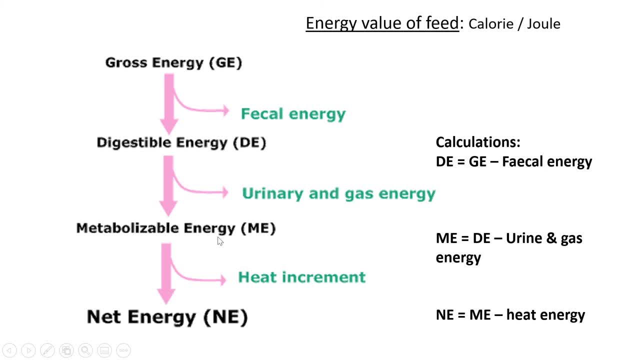 a little bit shorter. So the M-E metabolic energy. So to get the M-E you have to get the D-E. So you work from here. We already subtracted the fecal energy, So then you say D-E minus the urine energy and the gas energy. That gives you the M-E metabolic energy. 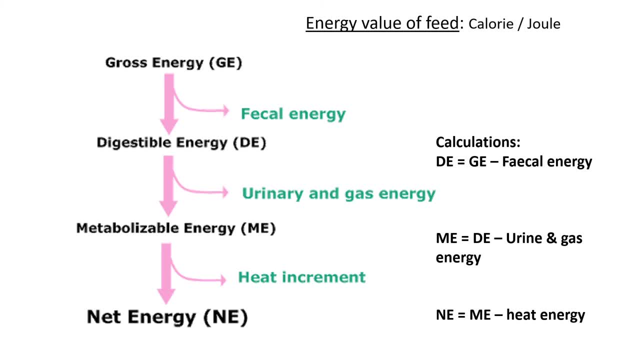 So I just want to mention: sometimes they either ask you, they give you the gross energy and they just ask you to get the net energy, So then you just simply minus all these things together, do one equation. But sometimes they ask you to figure out the D-E first and then to separately. 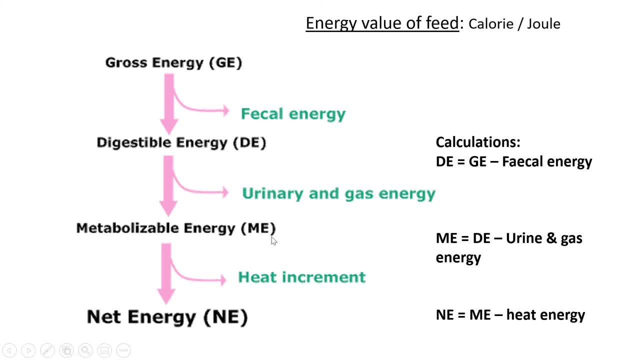 do the M-E afterwards, something like that. So that's why there are basically three equations here at the side. Depends on what they ask. So then you have to remember how to do this in sequence. So after you've got the M-E, then also energy will be lost through the skin of the animal. 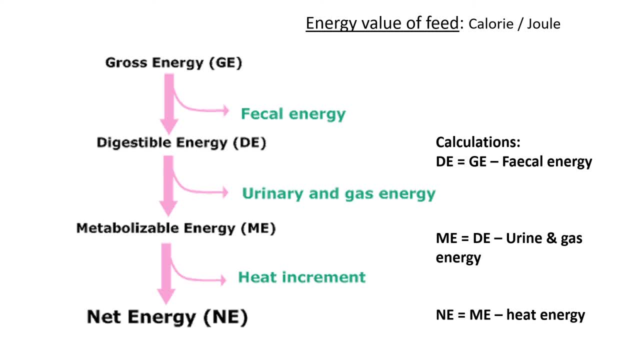 through heat energy, So meaning they respire or they sweat and so on, they lose heat through their skins. So then after that, if that is gone, you get net energy. So this is what the animal's left with at the end. 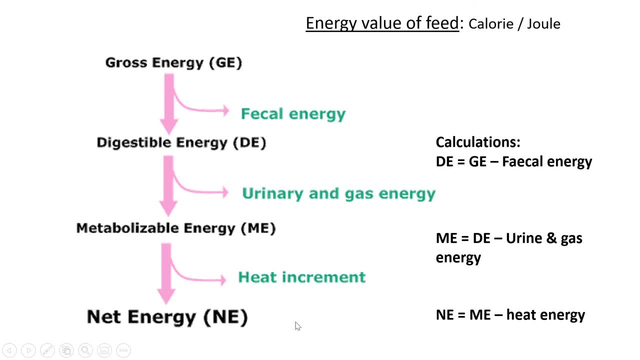 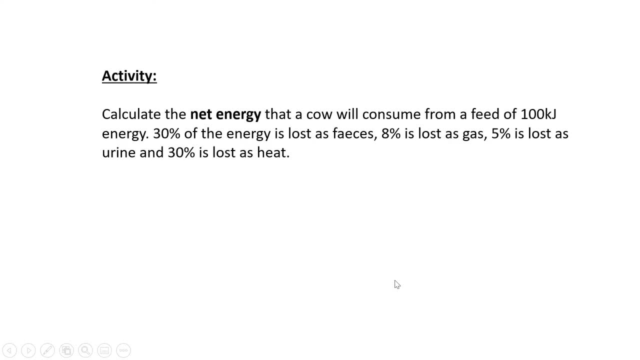 actually what they absorb or what they keep at the end. so the ne is then your me minus heat energy. okay, so here's an activity again. i recommend pause here, read through and then see if you can find the answer. answers on the next slide, actually just shortly. they ask you to calculate the net energy. 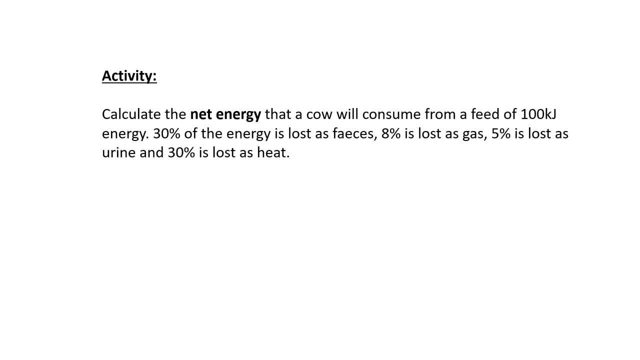 so this one is all the equations in one. that account will consume from the feet of 100 kilojoules energy. that's your gross energy. then 30 of the energy of the 100 is lost as feces, eight percent is lost as gas, five percent lost as urine and thirty percent lost as heat, and just a tip. 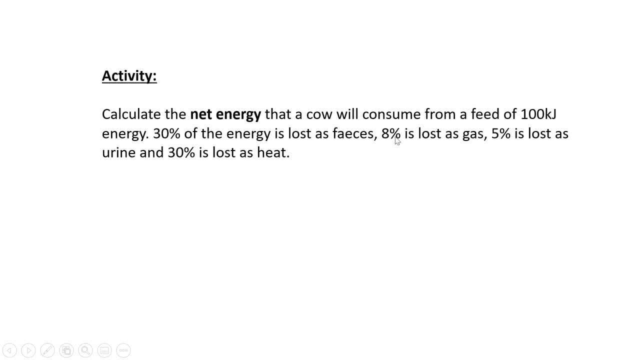 every time you figure out, or try to figure out, the kilojoules from the percentage go back to the original um amount of gross energy. so if you figure out the five percent it's gonna be five percent of a hundred, eight percent of a hundred, so on and so forth. 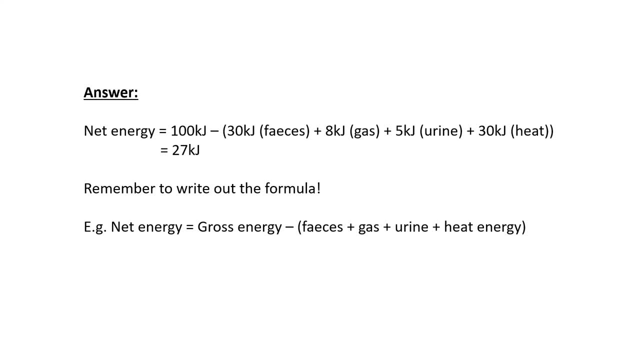 okay, so here's the answer. so basically, your net energy is your gross energy. let me just say the equation at the bottom here. then: net energy minus the gross energy, minus feces, plus gas, plus urine, plus use energy, all those energies together you minus from the gross energy and voila, you get the. 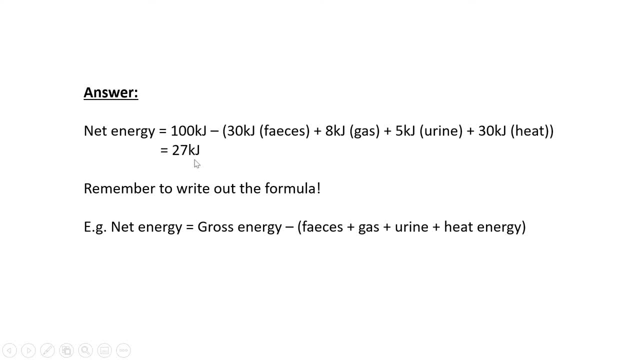 answer, and this is going to be 27 kilojoules. i just want to mention. if you compare this to 100 kgs, this is horrible. so this animal has lost so much energy just through feces and through its heat- body heat alone. so this would not be a good answer again anything. 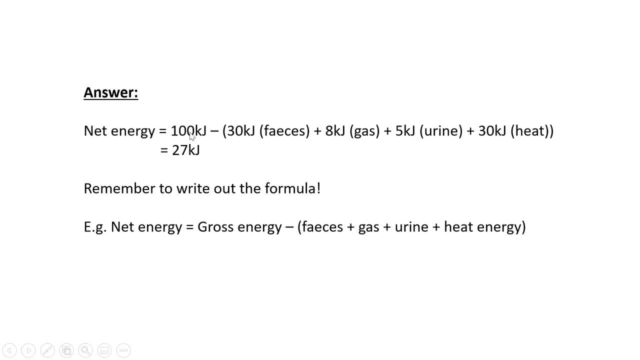 more than 50 percent. i want to say so, meaning over 50 kgs kilojoules- sorry, would be a good thing for me, it's about 50.. then also remember to write out the formula. you get a mark for the formula, even if you make up. 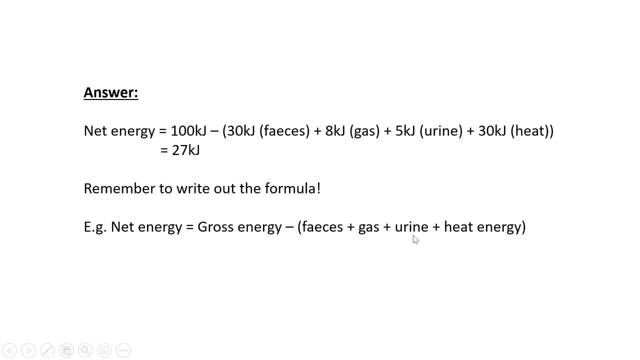 a formula like this. it's not exactly the formula we saw in the previous slide, doesn't matter, just as long as you indicated all the energies, in this case the net energy. i just included everything. i would not do it in three separate calculations or um equations. that's typical, that's also fine. okay, this last. 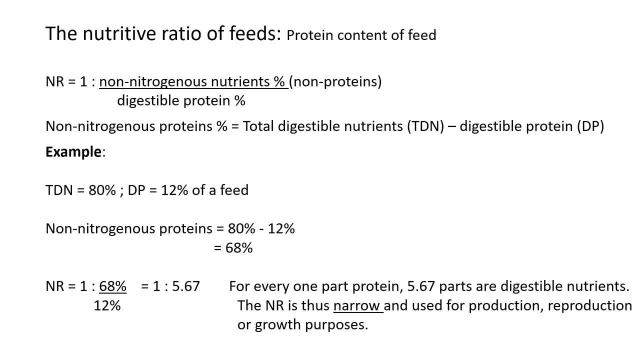 mention. sorry about this video, it's a little bit long. so the last thing is the nutritive ratio of feeds. in this case it also looks at the protein content of feeds. it's a lot like the bd value, but in this case you can actually do a calculation to figure it out. 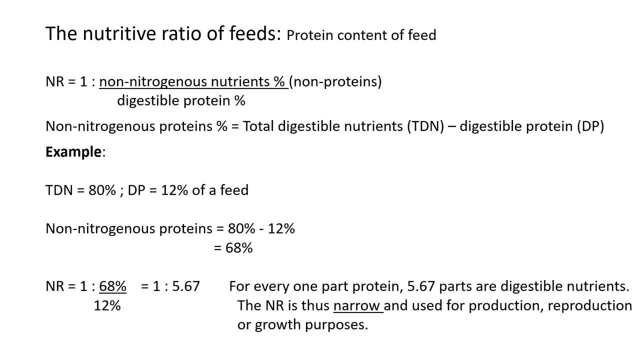 so the talked about the nr, so that it refers to the nutritive ratio and your equation at the top here is: the nr equals one to two non-mitogynous nutrients, so the non-proteins, everything that does not have proteins, like your vitamins, minerals, carbohydrates, fats, those. 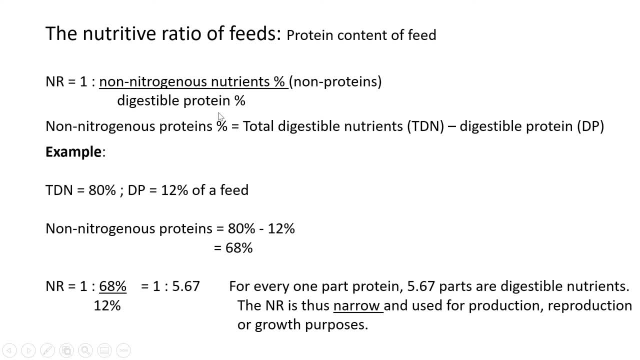 things divided by the usable protein, so all the protein percentage- and we work with percentage and this, by the way, the answer will also be: It'll be a ratio. So that's kind of what we're doing here. So the 1 indicates the amount of protein. 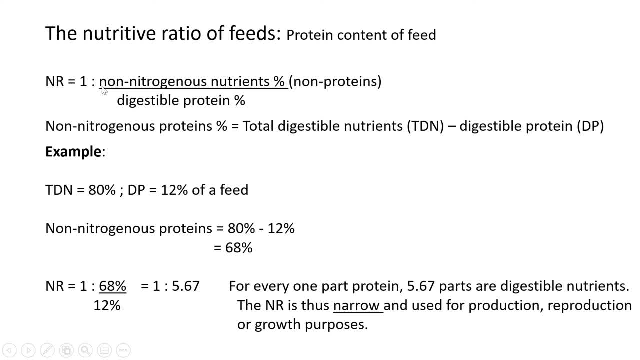 So it's going to be. this indicates protein, and whatever we write on this side is going to be the normal protein. So to figure out the non-itrogenous nutrients, you have to have the total digestible nutrients, called the TDM. You don't have to write out this entire thing. 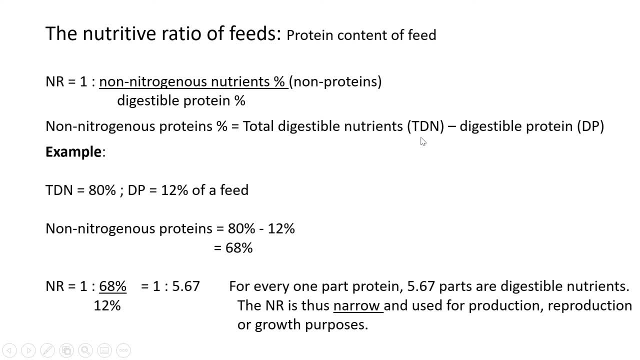 You can just say TDM, So that refers to the total digestible nutrients, which is everything, even the protein. So that's all nutrients, the animal ingests. Then you minus it with all the protein you have. So basically that gives you this the non-itrogenous nutrients. 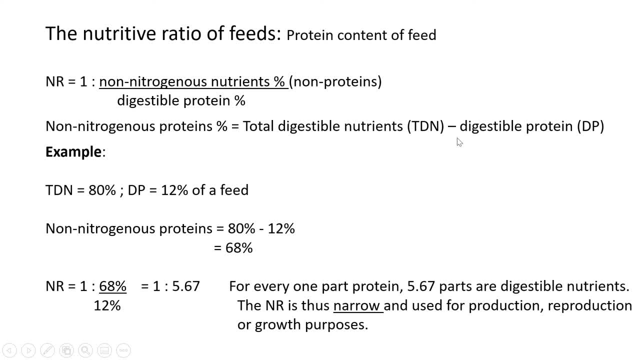 Usually they give you the TDM- all the nutrients the animal has absorbed- But you don't want to include the protein in there, because this side will include the protein. you want this side to be all about the non-protein. Okay, so just one example. 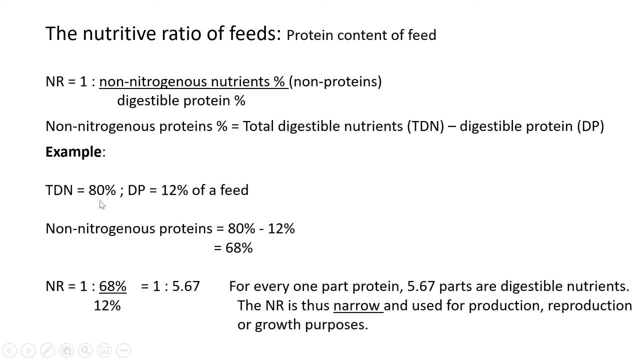 You're going to give us TDM as 80%, That's it. All your nutrients is 80% nutrients of what the animal absorbed or ingested. The protein is 12% of the feed. So to figure out what was not protein you have to say 80% minus the 12. 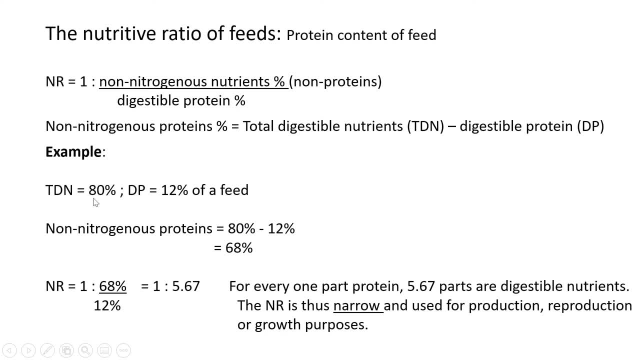 so 80% was basically nutrients the animal absorbed. We can assume the rest is maybe fiber and water. 12% was protein. 68% then was non-protein, So fats, carbs, anything else. So then you still have to put this into your equation. 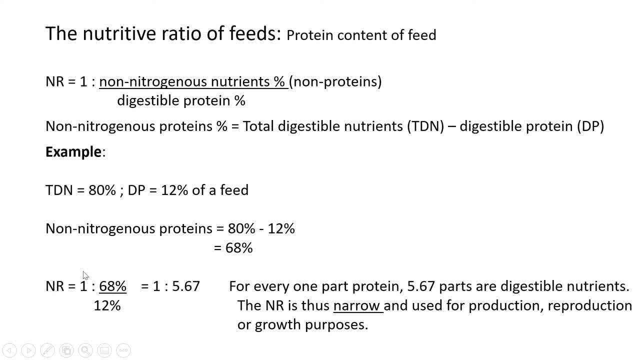 So then the NR nutritive ratio would be 1,. so one part protein to 68 over 12 non-nitrogen over your protein equals 1 to 5.67. So in this case you have one part protein and about six parts basically non-proteins. 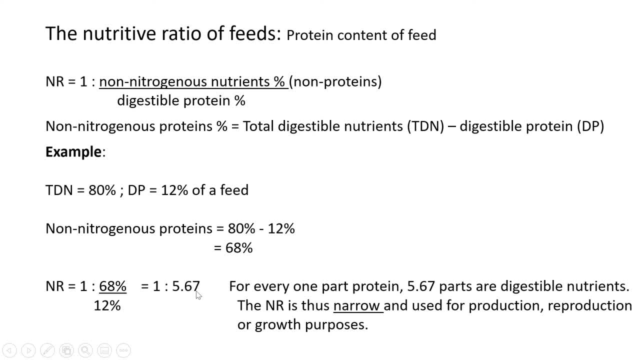 So meaning you're giving a lot of other types of nutrients to the animal and not a lot of protein. That's all right. That's basically what your ratio is. This is basically for a ration. What? What is the farmer doing? How much protein is he giving compared to everything else? 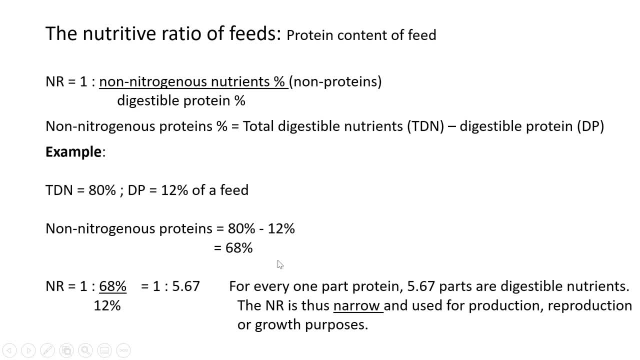 So that's trying to figure out the ration. So what does it mean in this case? For every one part protein, 5.67 parts are digestible nutrients. I mean everything else: fats, carbohydrates, so on. So the NR is in this case, narrow. 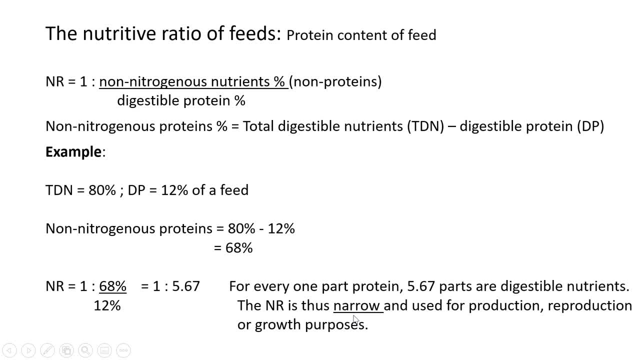 So you guys must be able to say whether it's narrow or wide. In this case it's narrow. Why? Because 5.67 is still less than 6. So if it's less this area less than 6, it's narrow. If it's more than 6, it's wide. 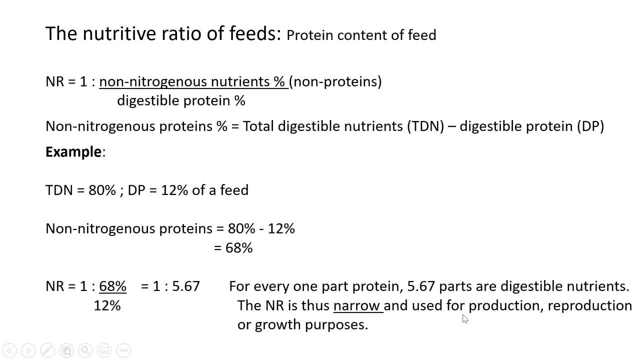 So in this case it's narrow and used for production, reproduction or growth purposes. So basically, when it's narrow, it means technically you're giving more protein Or a higher amount of protein compared to everything else, So it's still more non-protein you're giving. 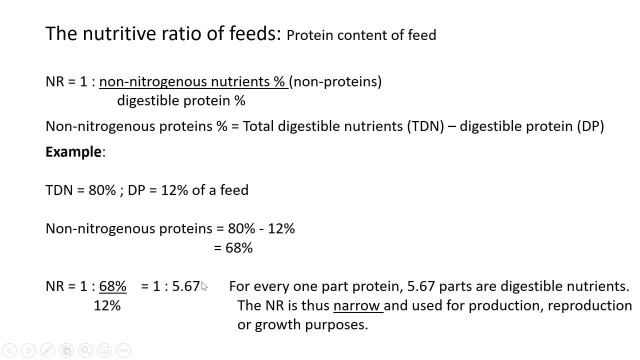 But in this case it's, I'm going to say, almost equal. it's not 1 to 1, but think of it that way: It's 5 is closer to 1 than, say, 6 or 9.. 9 is furthest away from 1. 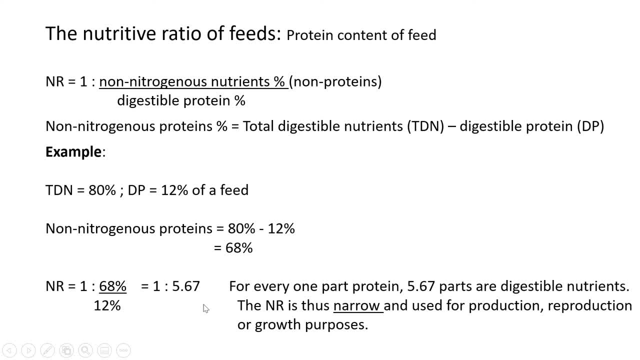 So you're giving a high amount of protein. That's the main idea. If it's 1 to 6 or 1 to 10, You're not giving a lot of protein, because that 10 indicates everything else. So then it's wide, meaning it's further away from the protein type. 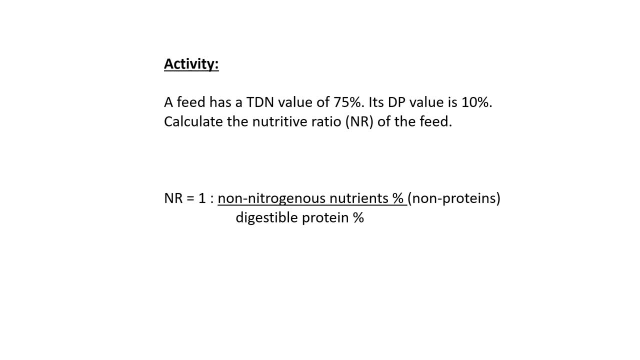 thing. Okay again, here's a nice activity. Pause again, because the answer is on the next slide. A feed has a TDN value of 75%. So that's all the nutrients: 75%. The protein content is 10%. Calculate the nutritive ratio of the feed and here's your formula again at the bottom: 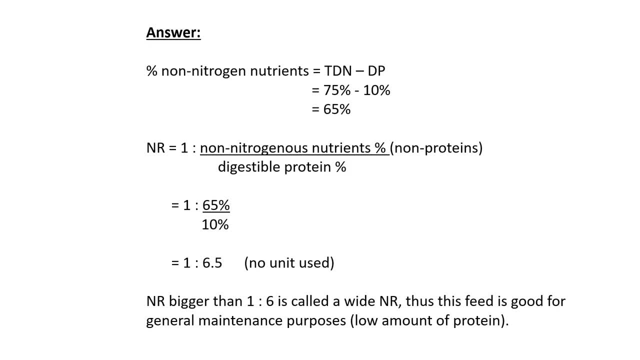 And here's your answer. So you say percent. you first have to figure out what is the non-nitrogen nutrient, so TDN minus TP, 75 minus 10, which is 65%. Then you can put that into your equation again. 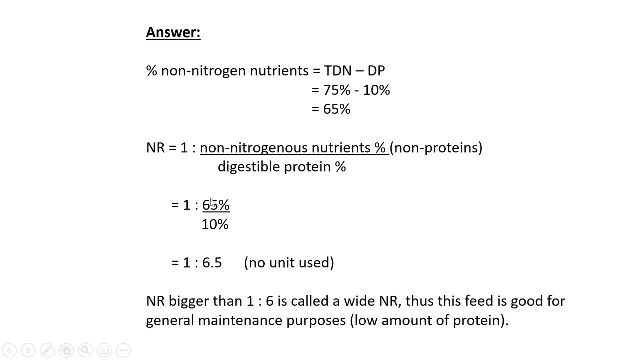 So that equals 1 to the 65 then is what is non protein? 10% is what does the protein? and it gives you 1 to 6.5, Again no units used, and in this case NR is bigger than 1.6 And that's called a wide NR. 6.5 is higher than 6.. So this feed is good for general maintenance.